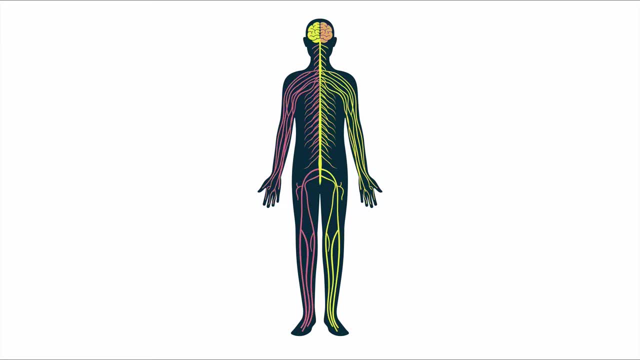 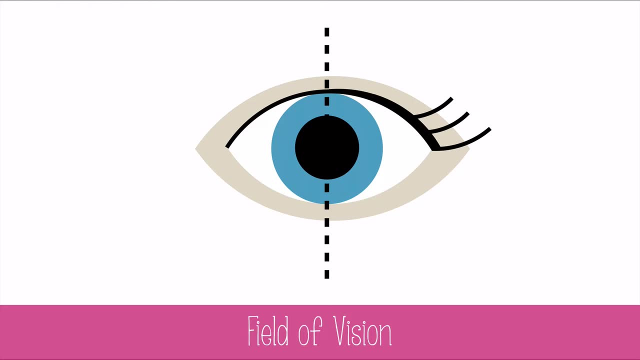 left side of the body and the left cerebral hemisphere receives sensory input from the right side of the body. In the eyes, the left field of vision for each eye is sent to the right visual cortex on the right occipital lobe and the right field of vision for each eye is sent to the 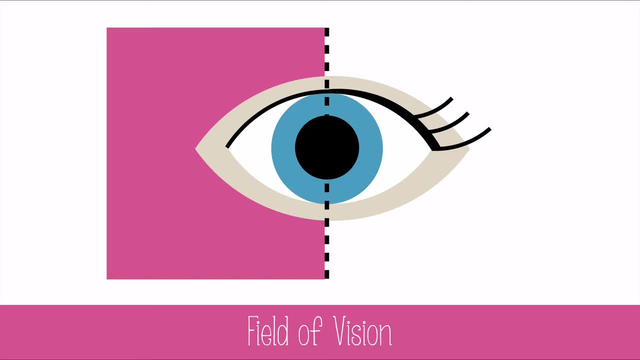 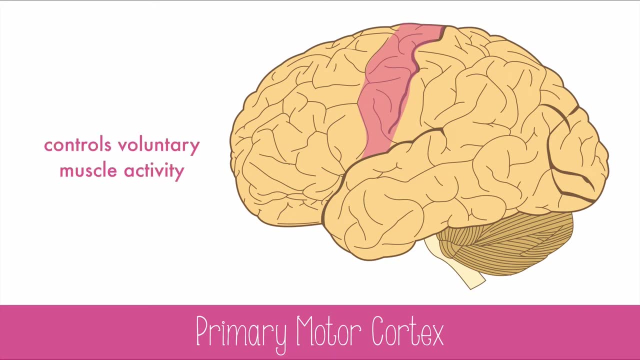 left visual cortex on the left occipital lobe. The part of the frontal lobes that controls muscle activity is called the primary motor cortex. The primary motor cortex in the left frontal lobe controls muscles on the right side of the body. The motor cortex on the right frontal lobe controls muscles on the left side of the body. 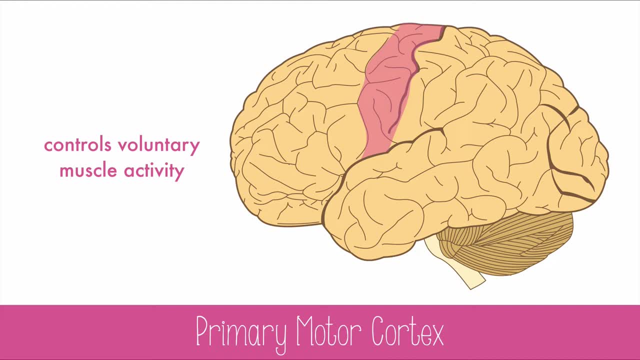 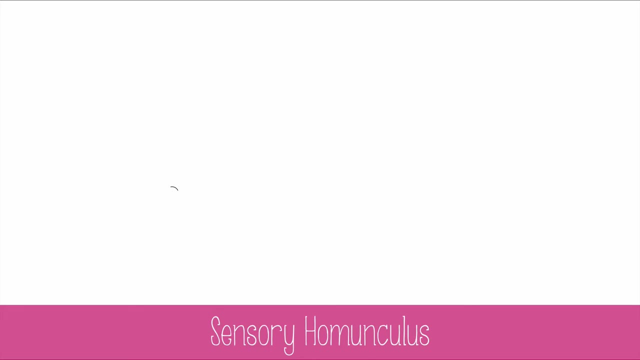 A stroke often paralyzes one side of the body. If the left side of the body has become paralyzed, this indicates the brain damage is actually in the right cerebral hemisphere, and vice versa. The major sensory and motor regions of the brain occupy the parietal and frontal lobes. 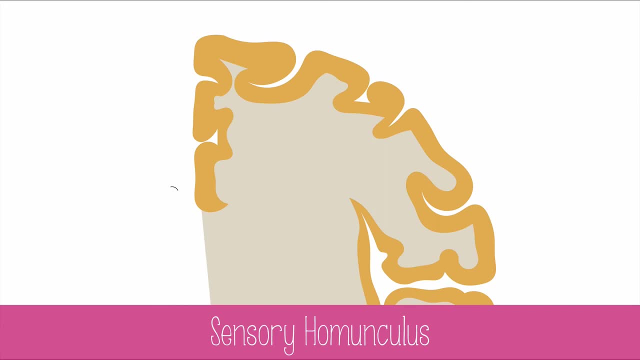 respectively. Studies have revealed that the brain does not dedicate space evenly to part of the body. The sensory homunculus shows how many nerves are dedicated to regions of the body by distorting the size of that body part. By the way, the word homunculus- 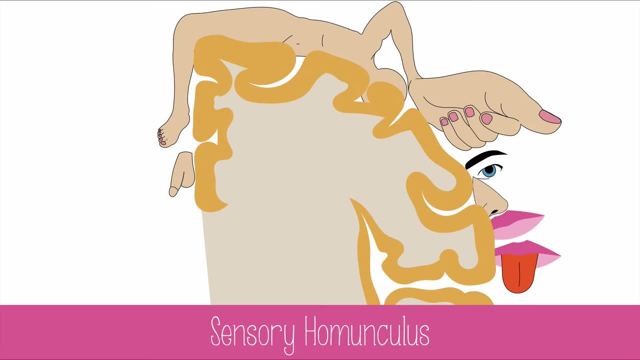 is just Latin for little man. You can see from this image that the hand is disproportionately large, which indicates that there are many nerves in the hand and much space dedicated to those neurons in the brain. The motor homunculus is similar to the sensory homunculus, with much innervation in the hands. 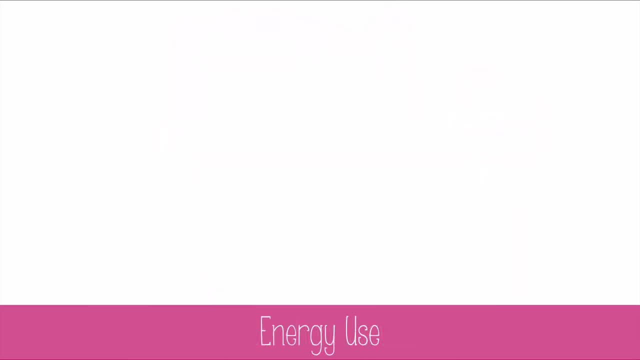 and face Our big thinking. brains use a huge amount of energy. About 20% of your body's energy at the basal metabolic rate is dedicated to the brain. Even more energy is dedicated to the brain in children. The reason for this goes back to how neurons actually send messages. 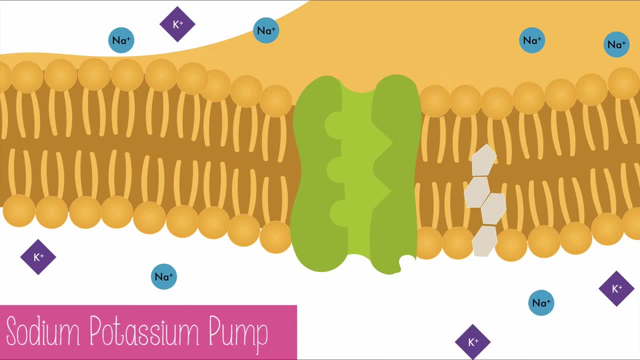 After each action potential, the sodium-potassium pump must use ATP to restore resting potential and move sodium back out and potassium back into the cell. This happens repeatedly along the axon of every neuron in the body. It should be no surprise that the brain uses so much energy. 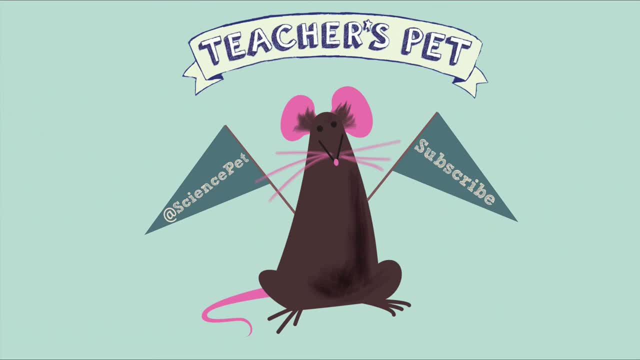 Thanks for watching this episode of Teacher's Pet. Don't forget to like and subscribe and follow me on Twitter at Science Pet.